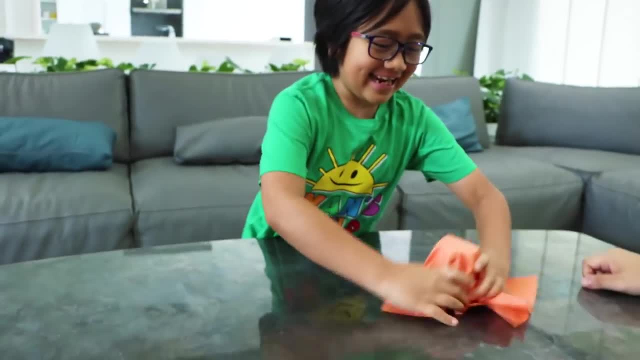 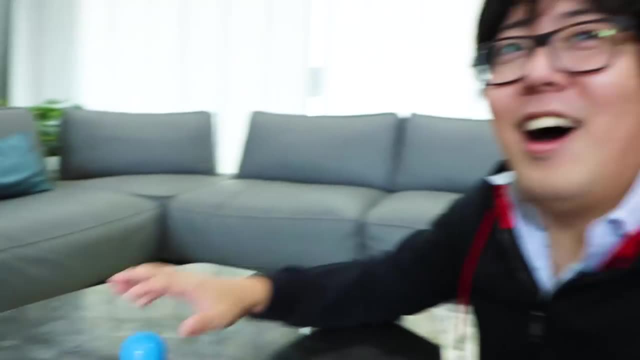 Did you not see it? I saw it. now He dropped it. And then, How come I didn't see it? Because I was making you look at this and not this. It's called misdirection. Oh Yeah, he got me good. 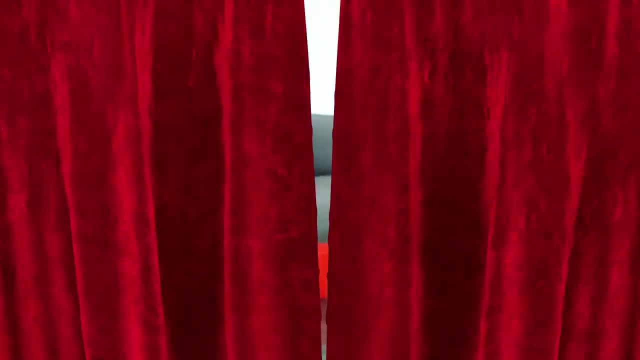 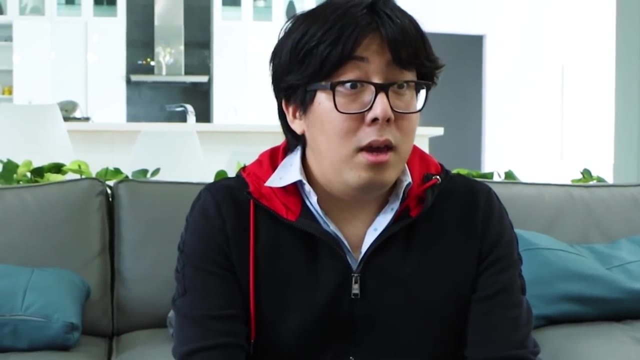 Can you beat that? I don't think I can beat that. Okay, Daddy, Show me what you got. Okay, so I have nothing in here and I have a cup. What I can do is make things appear and disappear. What kind of fruit do you like, Ryan? 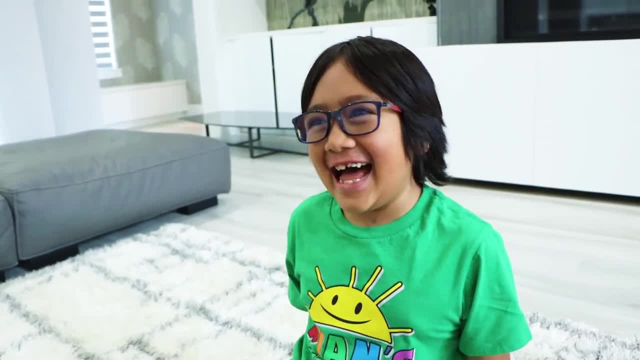 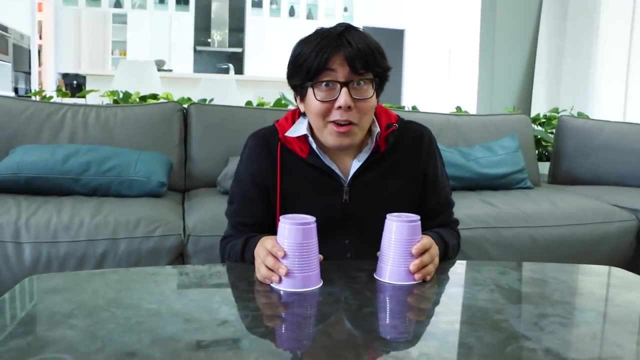 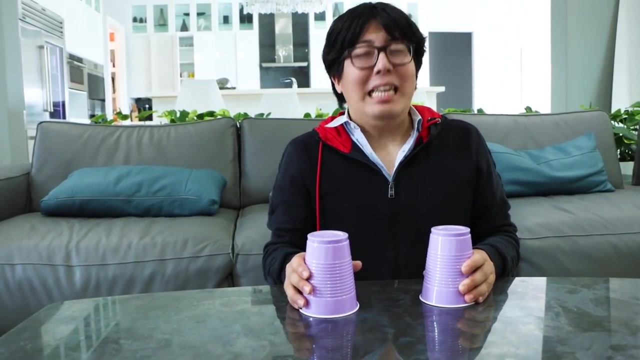 Good fruit, What kind of fruit? Orange. So I think Ryan said apple, I didn't hear orange. I'm going to make apple appear inside this cup. Actually, my hand can produce apples from nothing. Apples from nothing. Oops, I did too much. 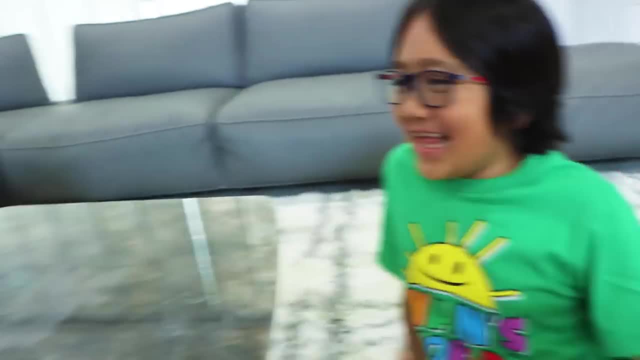 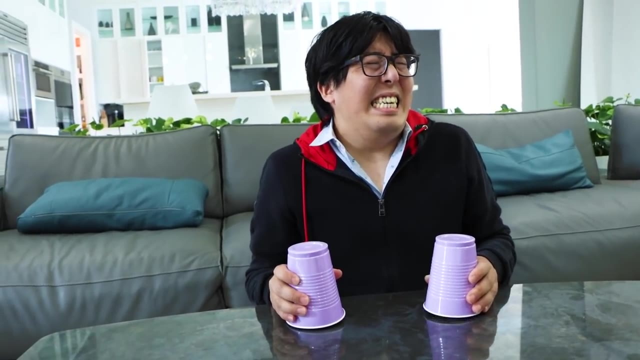 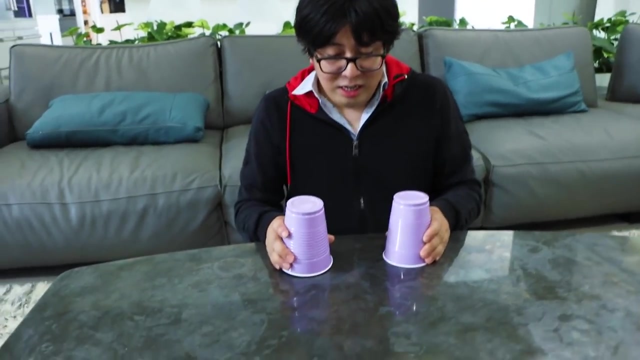 I got green apple, Small adjustment needed. Okay, I'm going to make this apple right here into the next cup. It's gone, right? What's that stuff? I saw some great stuff, though Apple here- Yeah, It's gone. 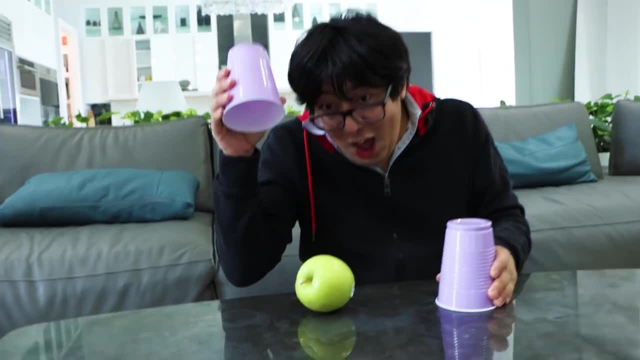 And I'm going to bring it over here. It's the magic. Okay, what about? No, no, no, This is off limit. You cannot touch the cup. It's very gentle. Do you guys know how I'm doing this? 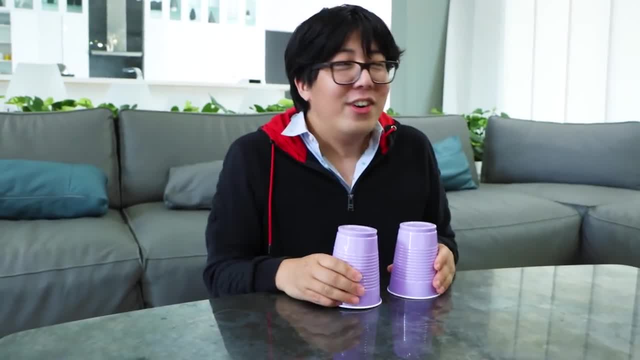 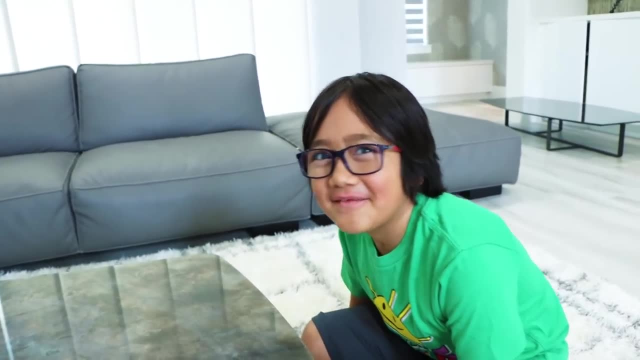 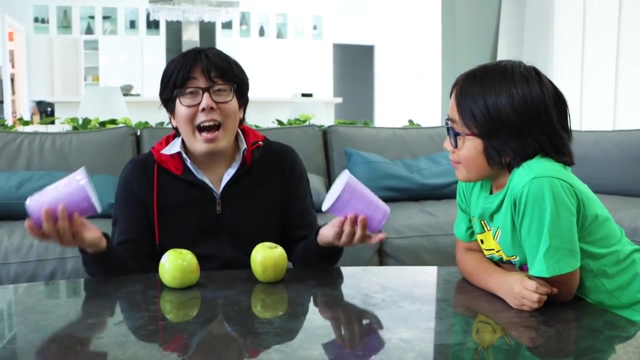 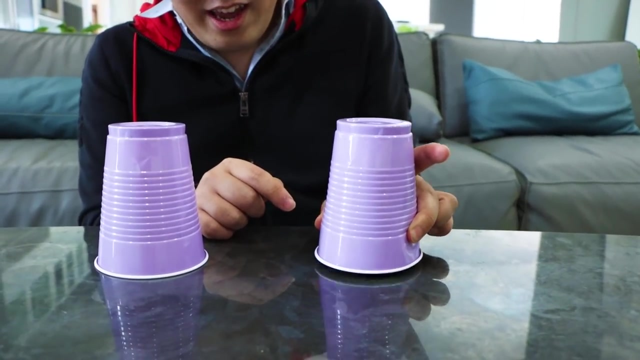 I wonder In here: Yeah, Both have apples? No, it's not there, See, Stop, Stop, All right. So what I did was I had apple the whole time inside the cup, but sometimes I hold the cup a little harder so I can grab the cup and apple inside together. 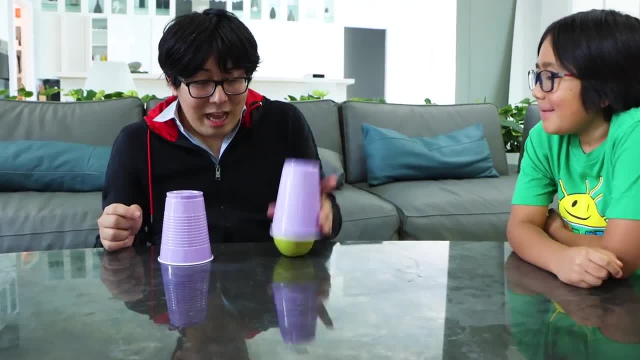 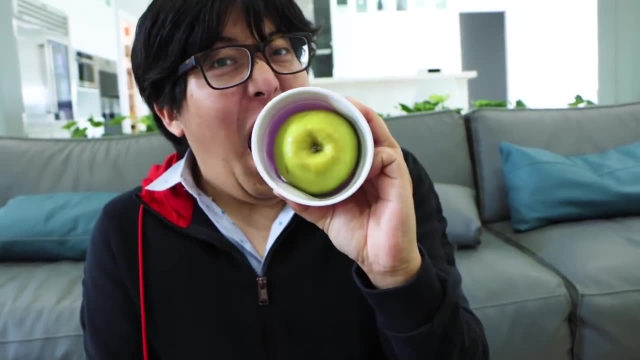 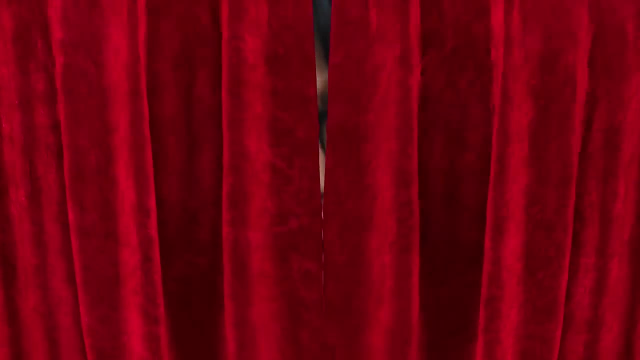 So sometimes apple there, not there, Here there, But you definitely don't want to show what's inside because the apple's still here. Okay, that's cool, Daddy, but I got another one for you. Okay, so I'm going to make this disappear when I put it inside the cup. okay,